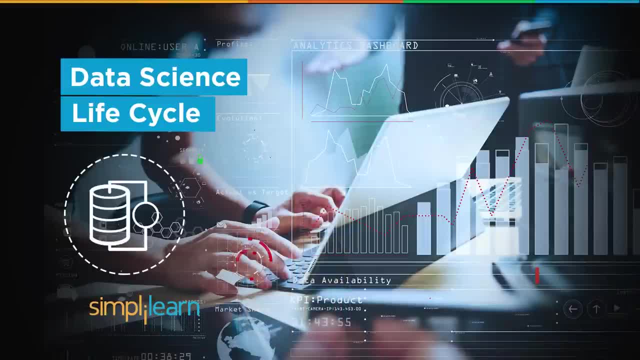 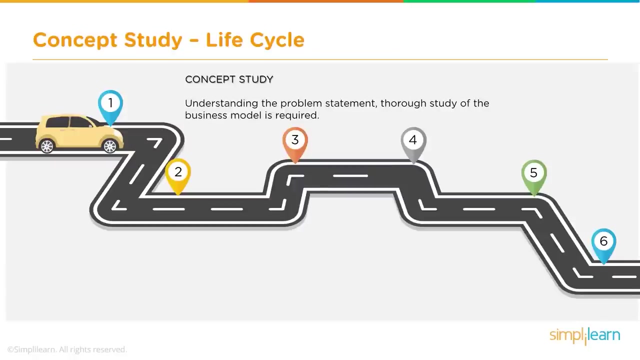 Hello and welcome to this session on data science. My name is Mohan and today we are going to take a look at what this buzz is all about. So now let's talk about the lifecycle of a data science project. Okay, the first step is the concept study. In this step, it involves understanding the business. 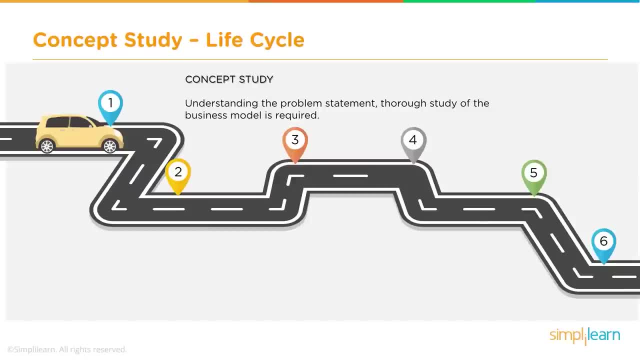 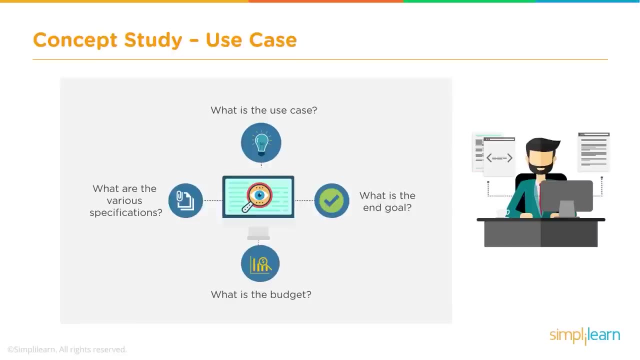 problem asking questions, get a good understanding of the business model, meet up with all the stakeholders, understand what kind of data is available, and all that is a part of the first step. So here are a few examples. We want to see what are the various specifications, and then what. 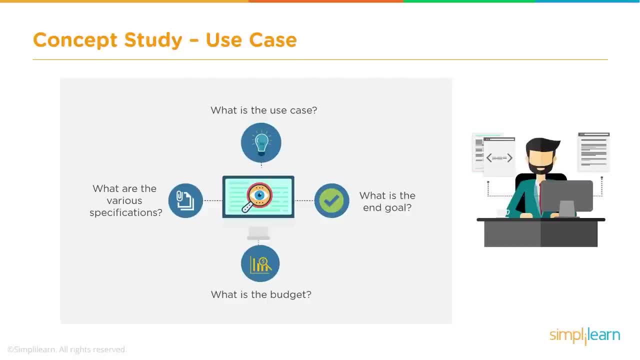 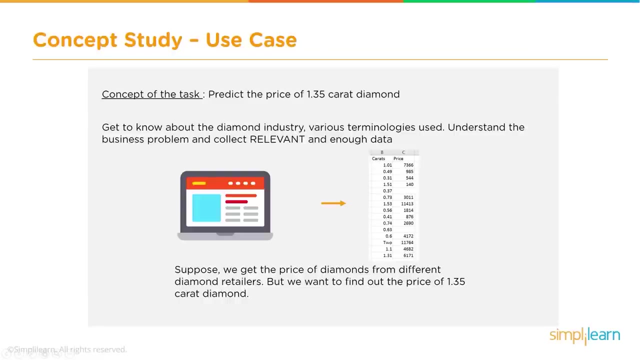 is the end goal? What is the budget? Is there an example of this kind of a problem that has been maybe solved earlier? So all this is a part of the concept study, And another example could be a very specific one: to predict the price of a 1.35 carat diamond. 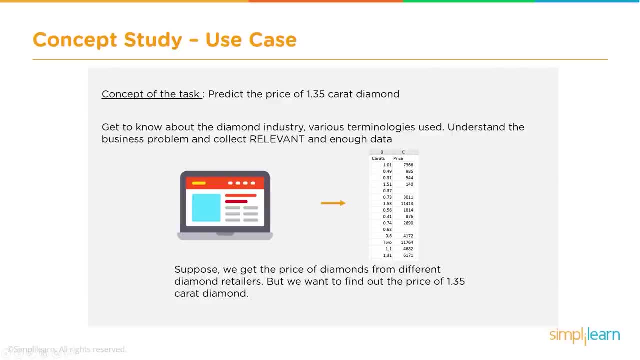 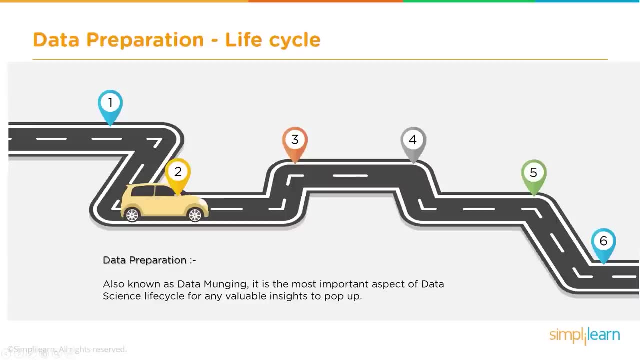 And there may be relevant information inputs that are available and we want to predict the price. The next step in this process is data preparation: data gathering and data preparation, also known as data munging, or sometimes it is also known as data manipulation. So what happens? 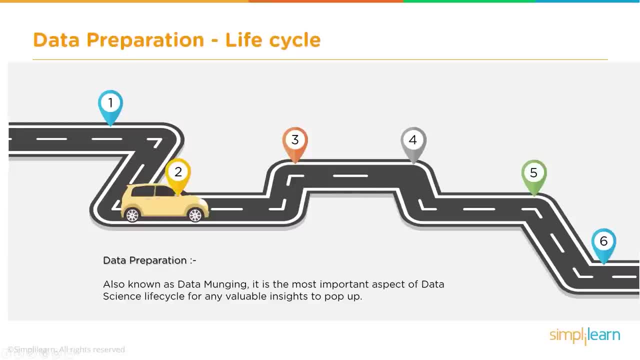 here is the raw data that is available. may not be usable in its current format for various reasons, So that is why, in this step, a data scientist would explore the data. He will take a look at some sample data, maybe pick. there are millions. 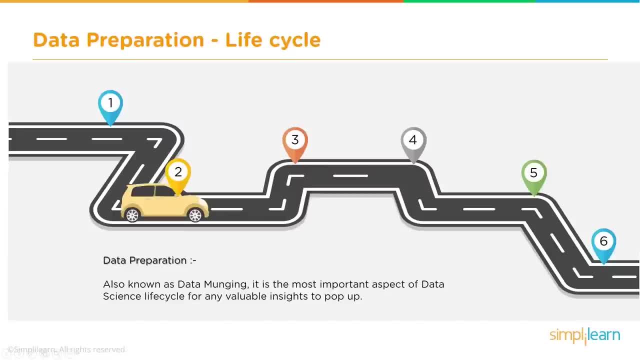 of records. pick a few thousand records and see how the data is looking. Are there any gaps? Is the structure appropriate to be fed into the system? Are there some columns which are probably not adding value may not be required for the analysis. Very often these are like: 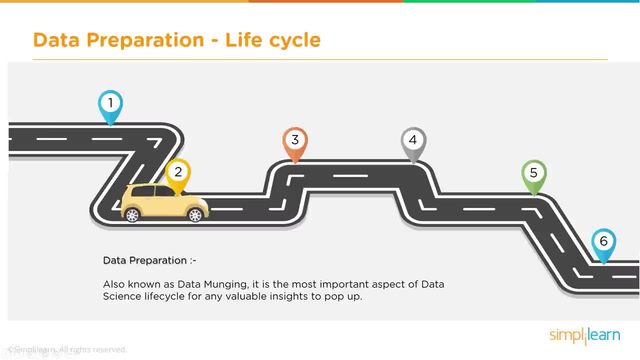 names of the customers. They will probably not add any value or much value from an analysis perspective. The structure of the data: maybe the data is coming from multiple data sources and the structures may not be matching. What are the other problems? There may be gaps in the data. 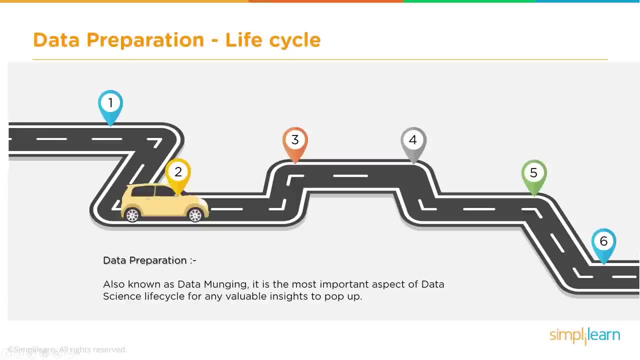 So the data, all the columns, all the cells are not filled. If you're talking about structured data, there are several blank records or blank columns. So if you use that data directly, you'll get errors or you'll get inaccurate results. So how do you either get rid of the data or how do you fill? 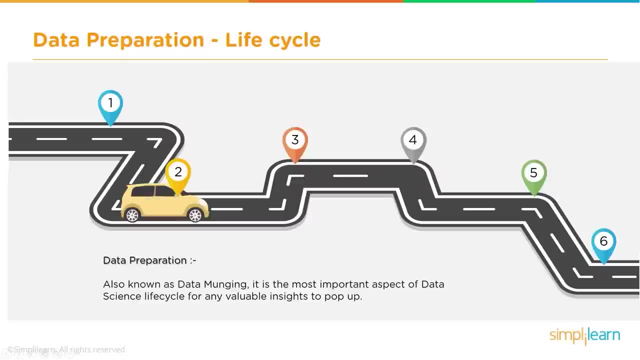 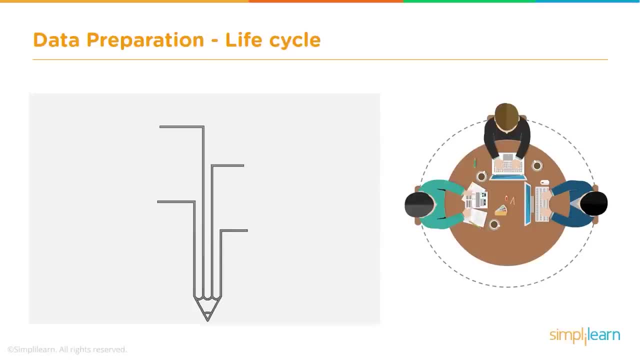 those gaps with something meaningful. So all that is a part of data munging or data manipulation. So these are some additional sub topics within that, So data integration is one of them. If there are any conflicts in the data there may be, data may be redundant, Yeah. 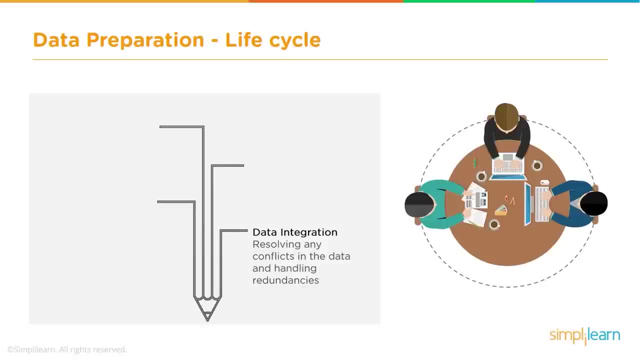 data redundancy is another issue There may be. you have, let's say, data coming from two different systems and both of them have customer table, for example, customer information. So when you merge them, there is a duplication issue. So how do we resolve that? So that is one. 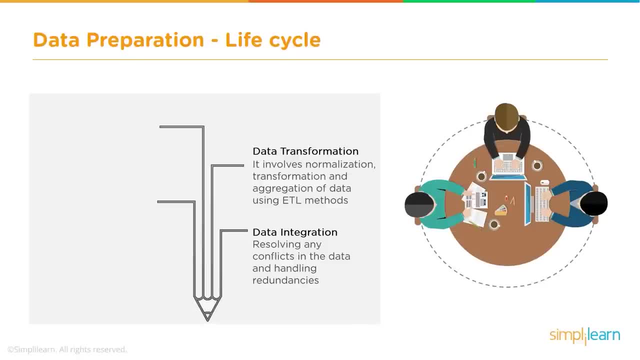 Data transformation. As I said, there will be situations where data is coming from multiple sources And then when we merge them together, they may not be matching. So we need to do some transformations to make sure everything is similar. We may have to do some data reduction. 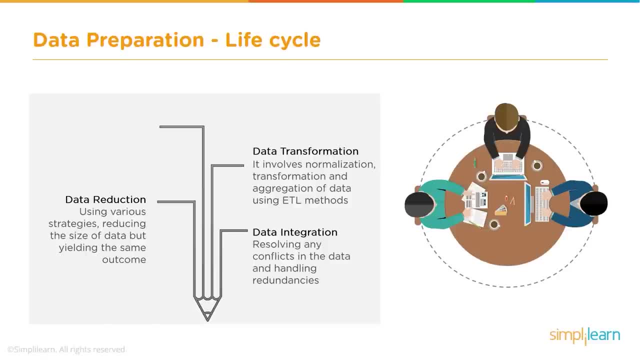 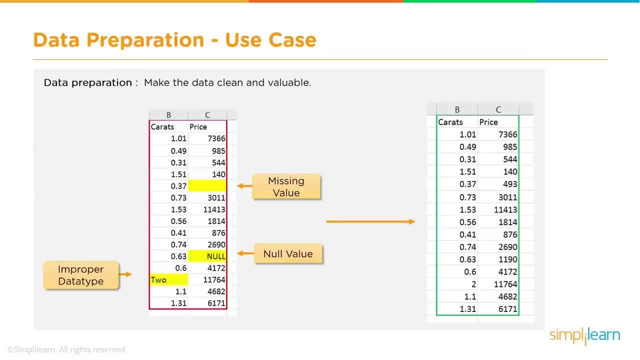 If the data size is too big, I have to come up with ways to reduce it meaningfully without losing information. Then data cleaning. So there will be either wrong values or null values, or there are missing values. So how do you handle all of that? A few examples of very specific stuff. So there are missing. 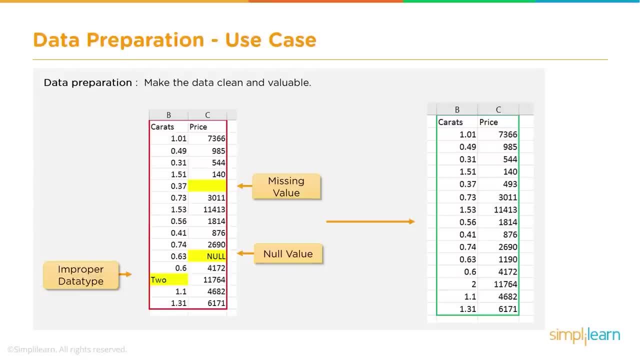 values. How do you handle missing values or null values Here? in this particular slide, we are seeing three types of issues. One is missing value, Then you have null value. You see the difference between the two right? So in the missing value there is nothing Blank Null value. it says null. Now the system cannot. 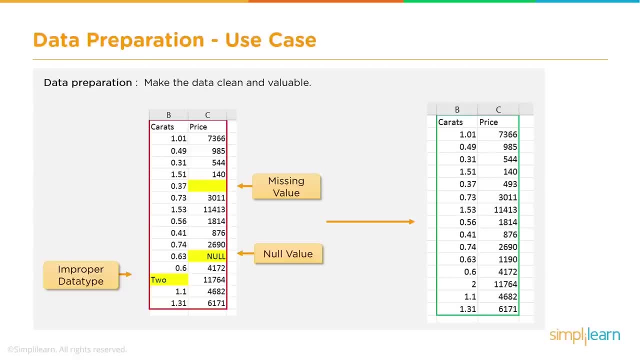 handle if there are null values? Similarly, there is improper data, So it's supposed to be numeric value, but there is a string or a non-numeric value. So how do we clean and prepare the data so that our system can work flawlessly? So there are multiple ways and there is no one. 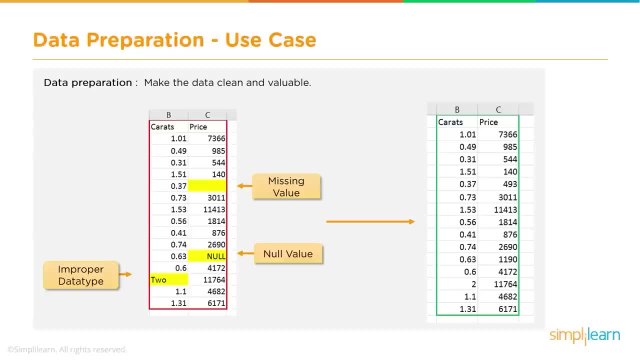 common way of doing this. It can vary from project to project. It can vary from what exactly is the problem we are trying to solve. So there are multiple ways to do this. So there are multiple ways to solve. It can vary from data scientist to data scientist, organization to organization. 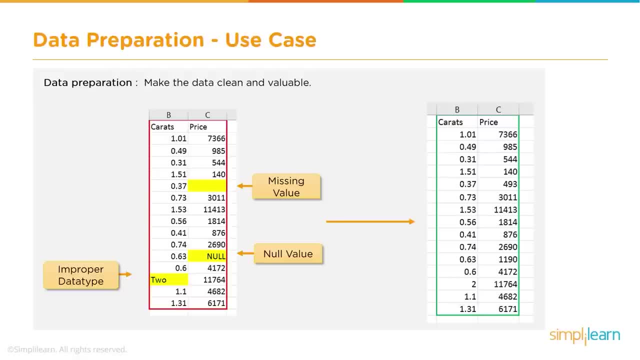 So these are, like some standard practices people come up with, And, of course, there will be a lot of trial and error. Somebody would have tried out something and it worked and will continue to use that mechanism, So that's how we need to take care of data cleaning. Now, what are the various ways? 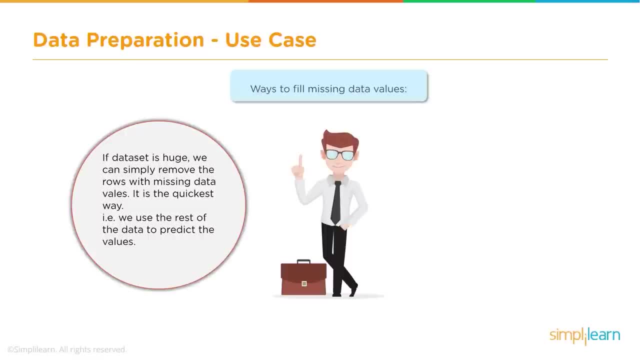 of doing. you know, if values are missing, how do you take care of that? Now, if the data is too large and only a few records have some missing value, then you have to take care of the data values. Then it is okay to just get rid of those entire rows, for example. So if you have a million, 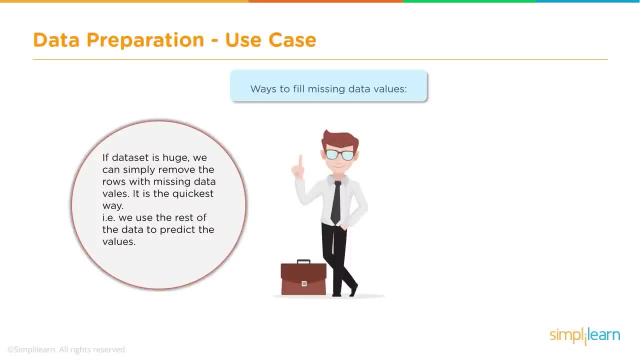 records and out of which 100 records don't have full data. So there are some missing values in about 100 records. So it's absolutely fine because it's a small percentage of the data, So you can get rid of the entire records which have missing values. But that's not a very common situation. 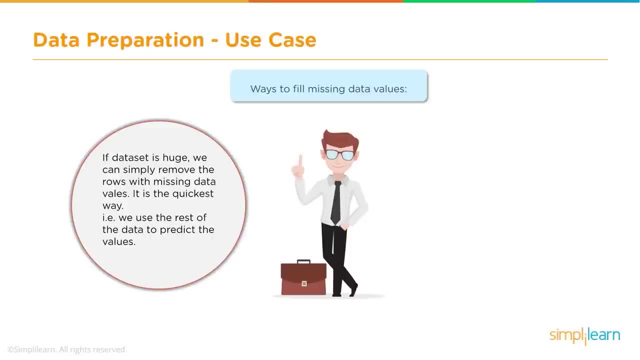 Very often you will have multiple or at least a large number of a data set. For example, out of 100 records, you may have 50,000 records, which are like having missing values. Now, that's a significant amount. You cannot get rid of all those records. Your analysis will be inaccurate. So how do you? 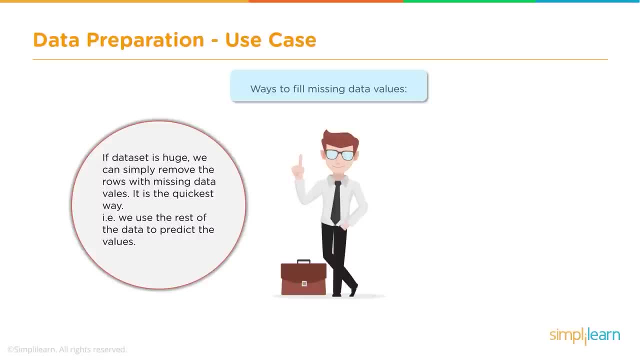 handle such situations. So there are again multiple ways of doing it. One is you can probably, if a particular values are missing in a particular column, you can probably take the mean value for that particular column and fill all the missing values with the mean value. So that, first of 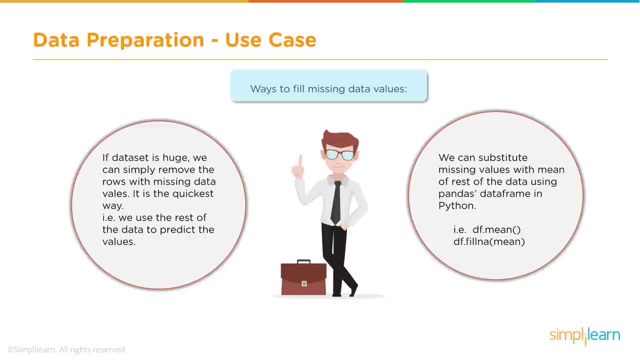 all, you don't get errors because of missing values And second, you don't get results that are way off because these values are completely different from what is there. So that is one way. Then a few other could be, either taking the median value or depending on what kind of data we are. 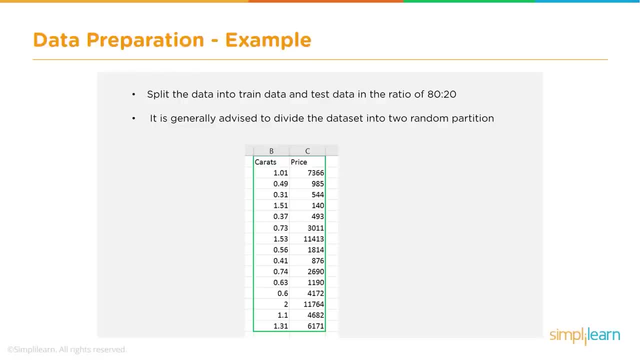 talking about, So something meaningful we will have put in there. If we are doing some machine learning activity, then obviously as a part of data preparation, you need to split the data into parts If you try to test with a data set which the system has already seen as a part of training. 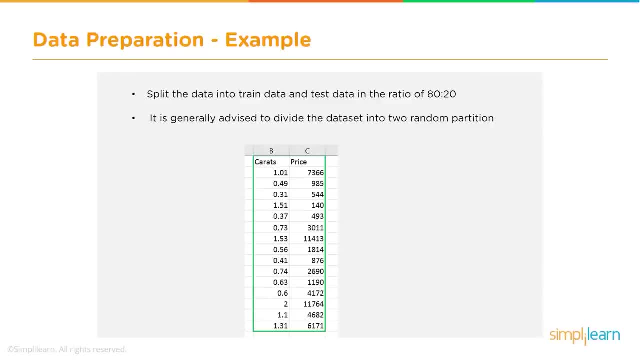 then it will tend to give reasonably accurate results because it has already seen that data And that is not a good measure of the accuracy of the system. So typically you take the entire data set, the input data set, and split it into two parts, And again the ratio can vary from person to person. 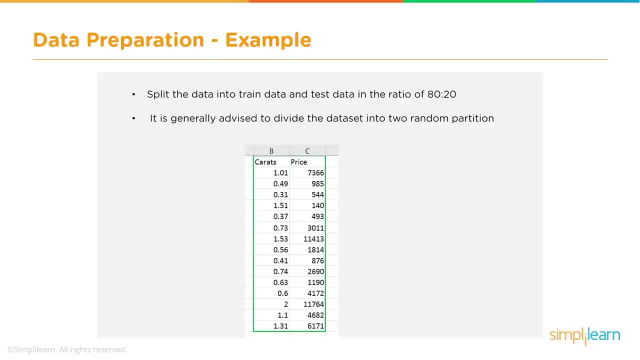 individual preferences. Some people like to split it into 50- 50.. Some people like it as 63.33 and 33.3 is basically two third and one third. And some people do it as 80, 20, 80 for training and 24 testing. So you split the data, perform the training with the 80% and then use. 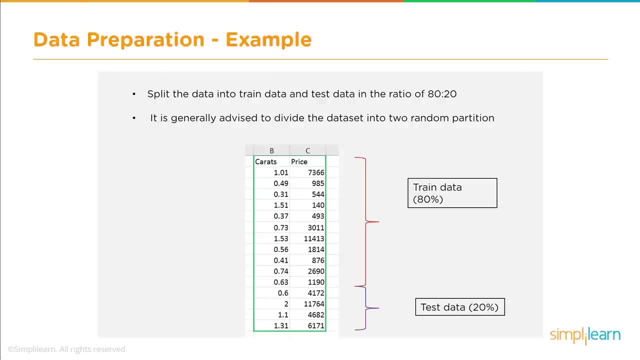 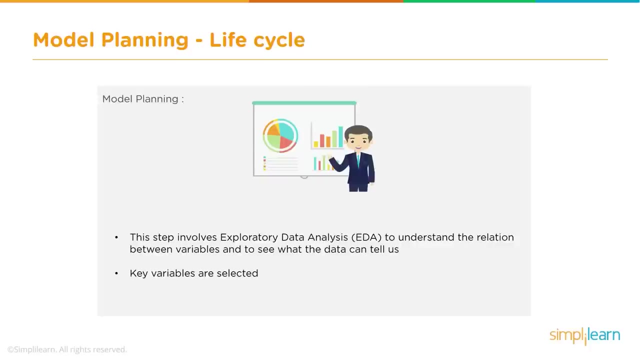 the remaining 20% for testing, All right. So that is one more data preparation activity that needs to be done before you start analyzing or applying the data or putting the data through the model. Then the next step is model planning. Now this models can be statistical models. This could be machine learning models. 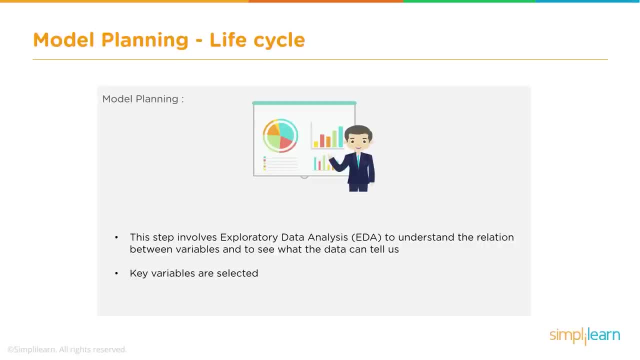 So you need to decide what kind of models you're going to use. Again, it depends on what is the problem you're trying to solve. If it is a regression problem, you need to think of a regression algorithm and come up with a regression model. So it could be linear regression Or if 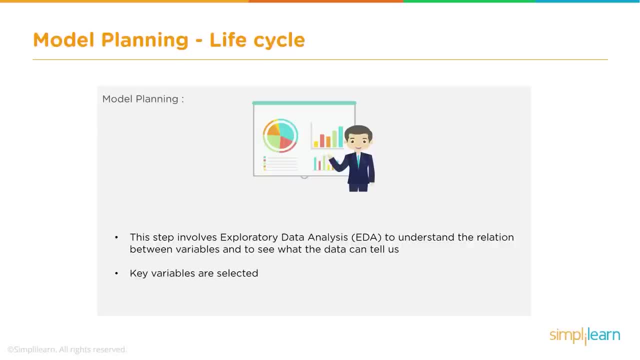 you are talking about classification, then you need to pick up an appropriate classification algorithm, like logistic regression or decision tree or SVM, And then you need to train that particular model. So that is the model building or model planning process, And the cleaned up data has to be fed into the model. And, apart from cleaning, 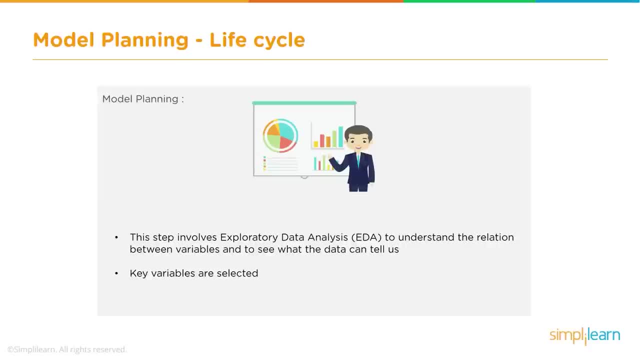 you may also have to. in order to determine what kind of model you will use, you have to perform some exploratory data analysis to understand the relationship between the various variables and see if the data is appropriate, and so on. Right, So that is the. 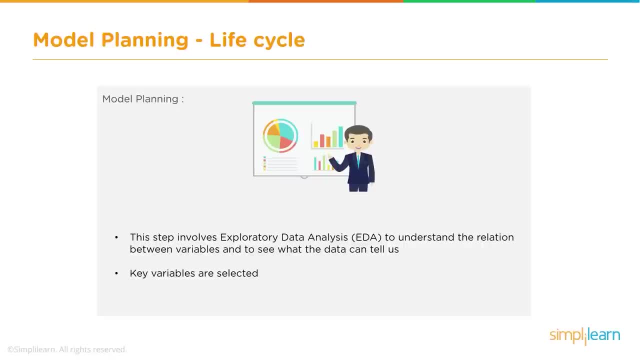 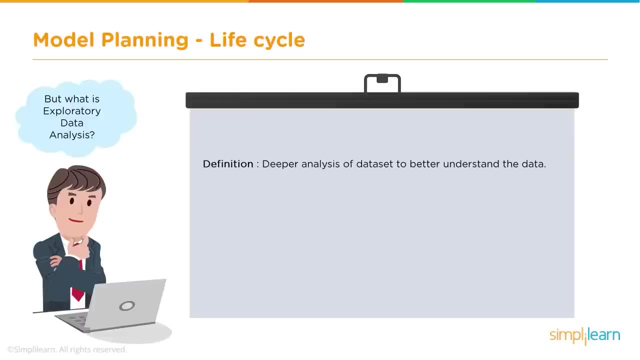 Additional preparatory step that needs to be done. So little bit of details about exploratory data analysis. So what exactly is exploratory data? analysis is basically to, as the name suggests, you're just exploring. you just receive the data and you're trying to explore and find out what. 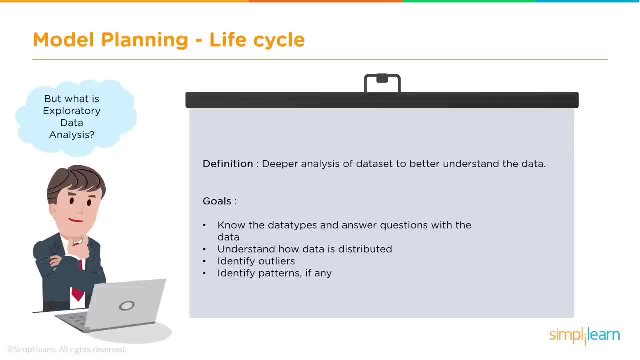 are the data types and what is the? is the data clean in in each of the columns? what is the maximum minimum value? So, for example, there are out of the box functionality available in tools like R. So, if you just Ask, 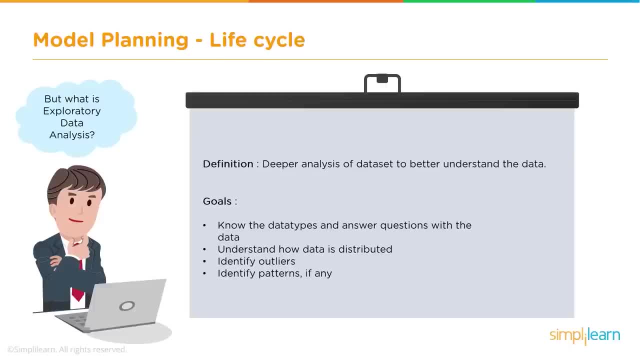 For a summary of the table. it will tell you for each column, it will give some details as to what is the mean value, what is the maximum value, and so on and so forth. So this exercise, or this exploratory analysis, is to get an understanding of your data And then 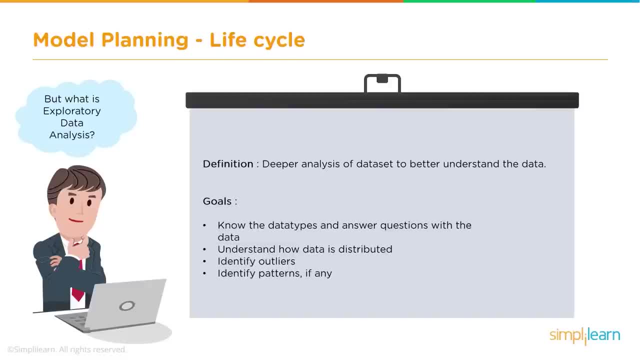 you can take steps to. during this process, you find there are a lot of missing values. You need to take steps to fix those. You will also get an idea about what kind of model to be used, and so on and so forth. What are the various techniques used for exploratory data analysis? 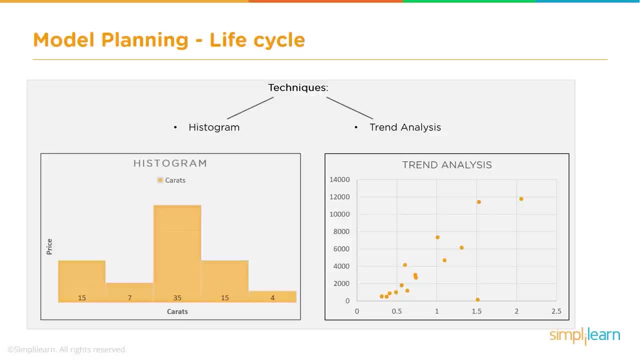 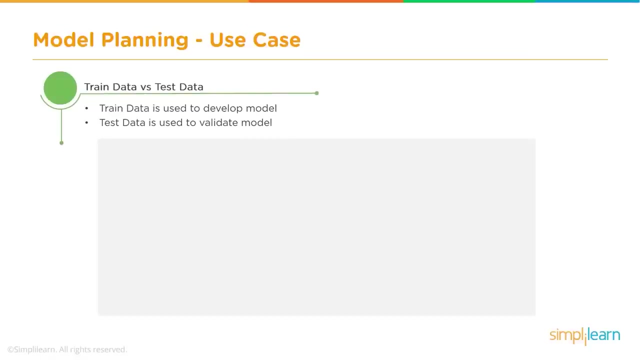 Typically these would be visualization techniques. like you use histograms, you can use box plots, you can use scatter plots, So these are very quick ways of identifying the patterns or a few of the trends of the data and so on. And then, once your data is ready, you decided on the model. 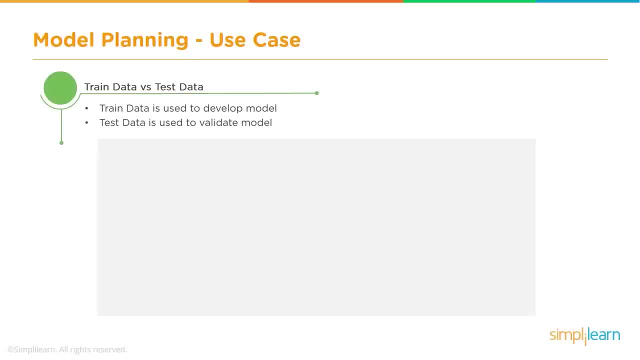 what kind of model, what kind of algorithm you're going to use. If you're trying to do machine learning, you need to pass your 80% the training data. or rather, you use that training data to train your model And the training process itself is iterative. So for the training process, 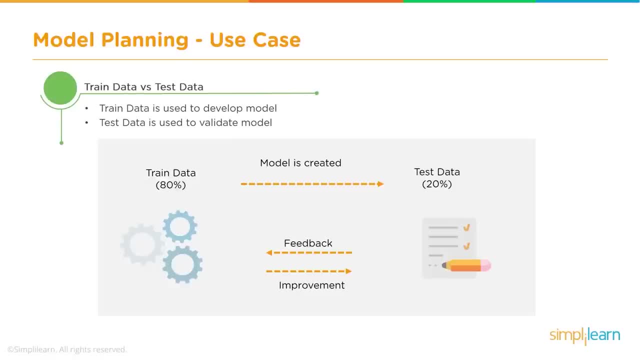 you may have to perform multiple times, And once the training is done and you feel it is giving good accuracy, then you move on to test. So you take the remaining 20% of the data. Remember, we split the data into training and test, So that test data is now used to check the 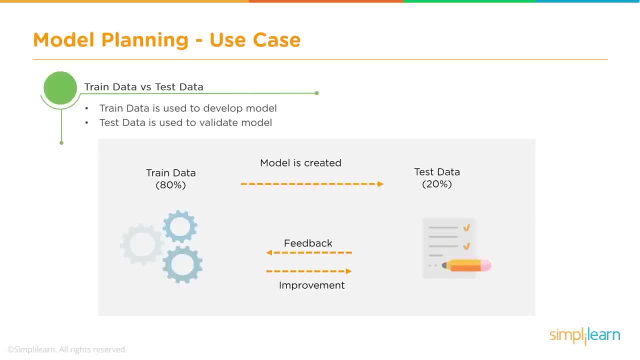 accuracy or how well our model landscape is going to perform, how well the model is planned model is performing. And if there are further issues- let's say the model is still during testing and the accuracy is not good- then you may want to retrain your model or use a different. 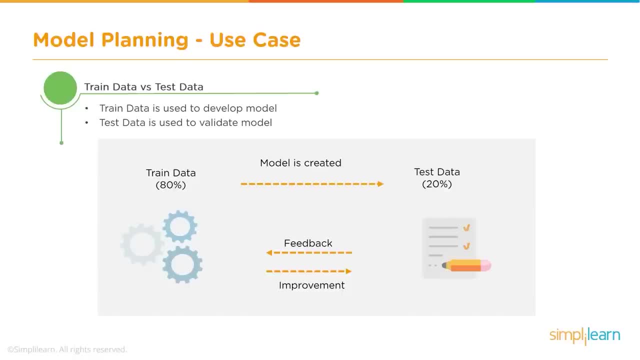 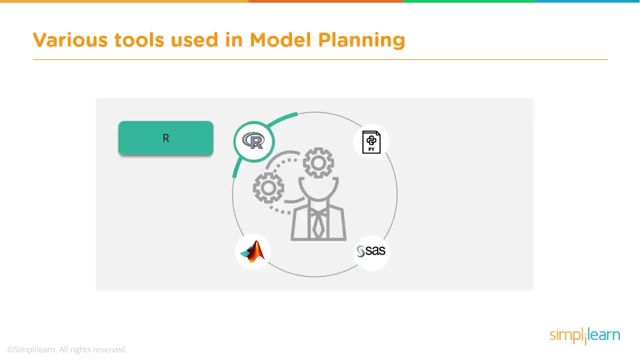 model. So this whole thing again can be iterated. But if the test process is passed, or if the model passes the test, then it can go into production and it will be deployed. All right, So what are the various tools that we use for model planning? R is an excellent tool in a lot of ways, whether 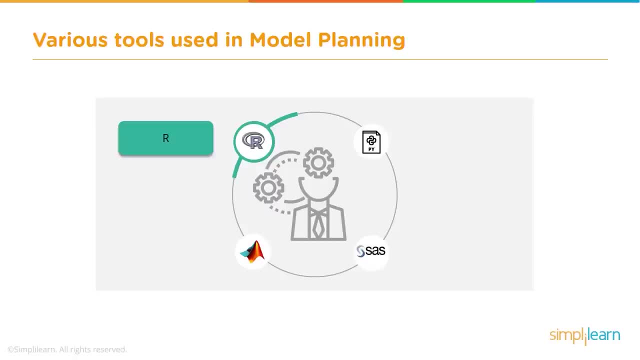 you're doing regular statistical analysis or machine learning or any of these activities. R, along with RStudio, provides a very powerful environment to do data analysis, including visualization. It has a very good integrated visualization or plot mechanism which can be used for doing exploratory data analysis and then later on to do 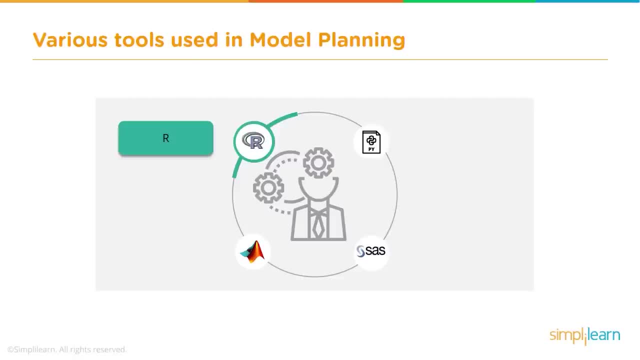 data analysis, Analysis, detailed analysis and machine learning, and so on and so forth. Then, of course, you can write Python programs. Python offers a rich library for performing data analysis and machine learning, and so on. MATLAB is a very popular tool as well, especially during education, So this is. 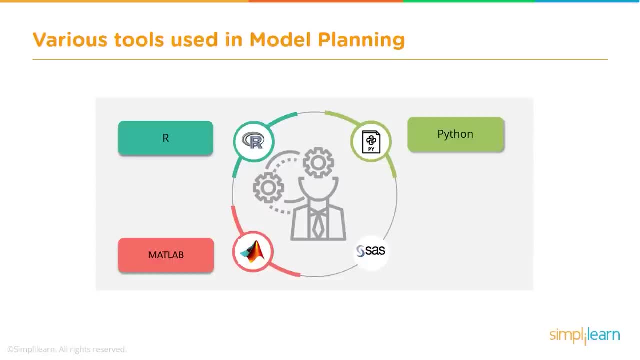 a very easy to learn tool. So MATLAB is another tool that can be used. And then, last but not least, SAS. SAS is again very powerful. It is a proprietary tool And it has all the components that are required to perform very good statistical analysis or perform 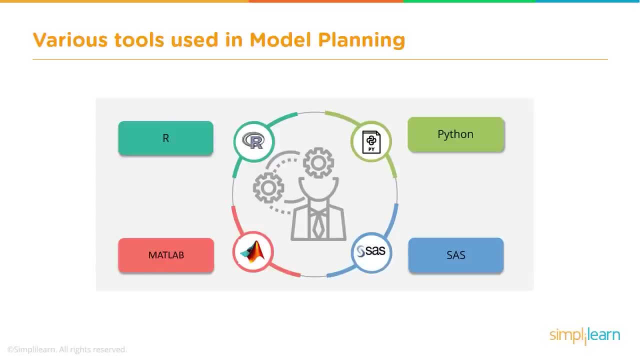 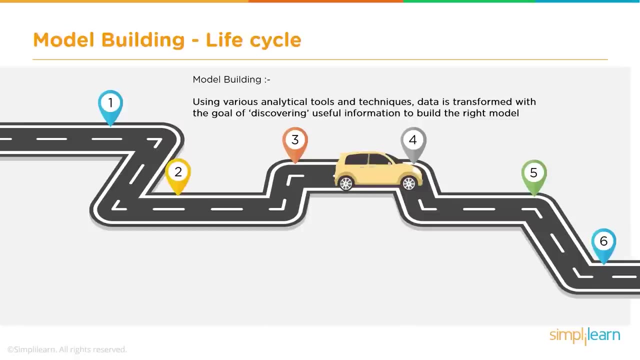 data science. So those are the various tools that would be required for, or that that can be used for, model building, And so the next step is model building. So we have done the planning part. We said, OK, what is the algorithm we are going to use, What kind of model we are going to use? 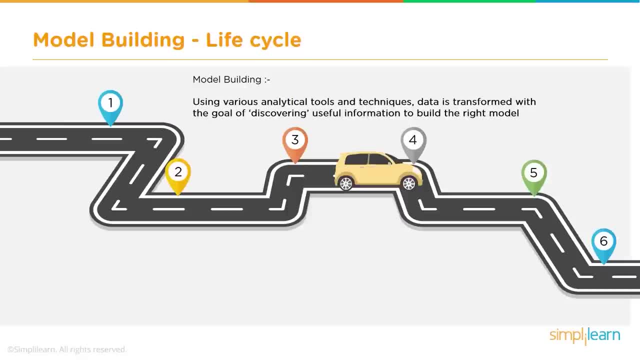 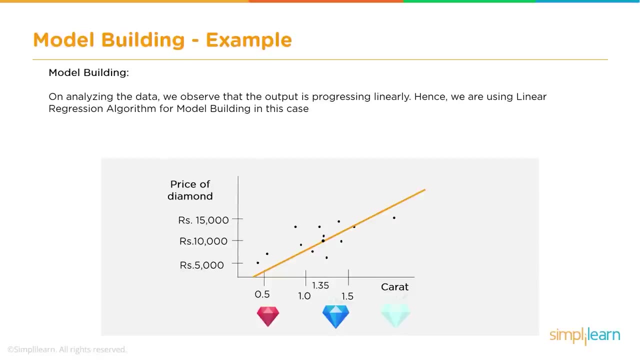 Now we need to actually train this model, or build the model, rather, so that it can then be deployed. So what are the various ways or what are the various types of model building activities? So it could be, let's say, in this particular example that we have taken, you want to find out? 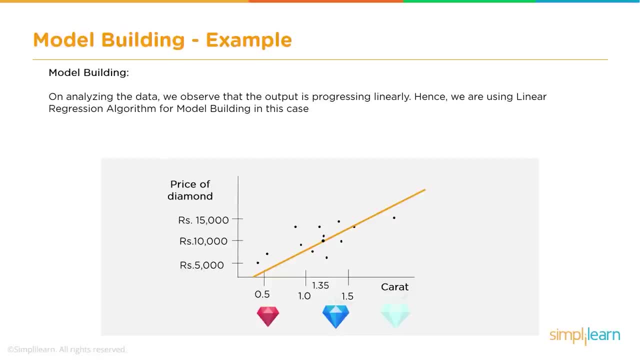 the price of 1.35 carat diamond. So this is, let's say, a linear regression problem. You have data for various carats of diamond and you use that information. You pass it through a linear regression model or you create a linear regression model. 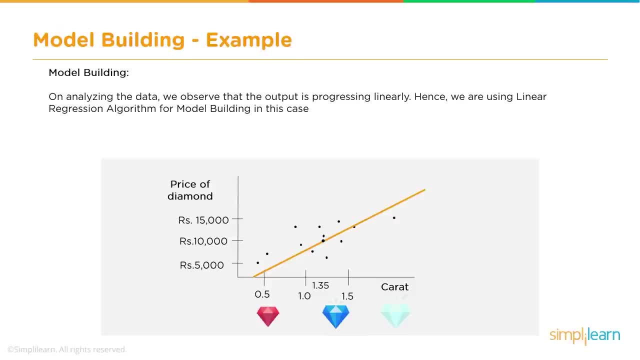 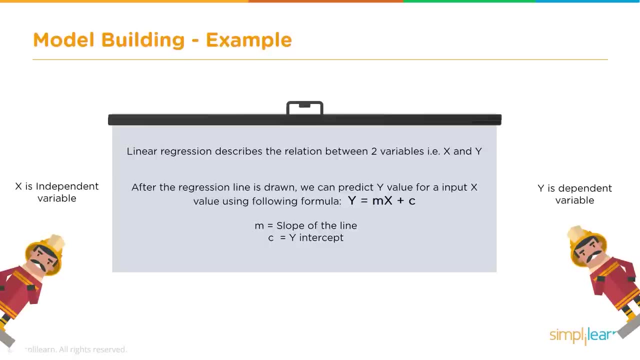 Which can then predict your price for 1.35 carat. So this is one example of model building and then a little bit details of how linear regression works. So linear regression is basically coming up with a relation between an independent variable and a dependent variable. So it is pretty much. 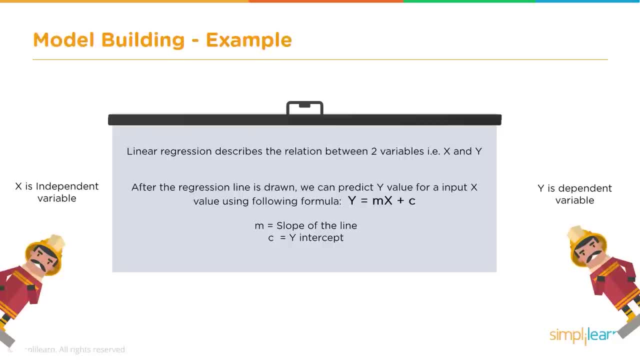 like coming up with equation of a straight line which is the best fit for the given data. So like, for example here: y is equal to mx plus c, So y is the dependent variable and x is the independent variable. We need to determine the values of m and c for our given data. So that is what the training 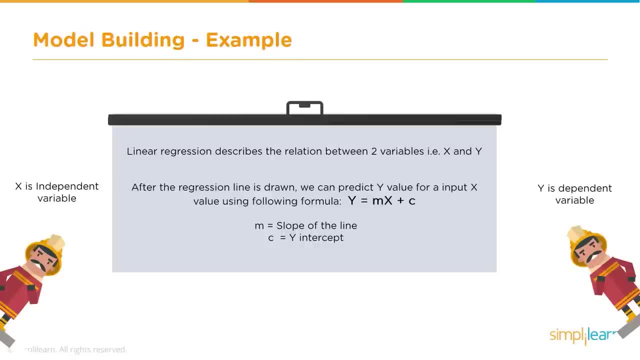 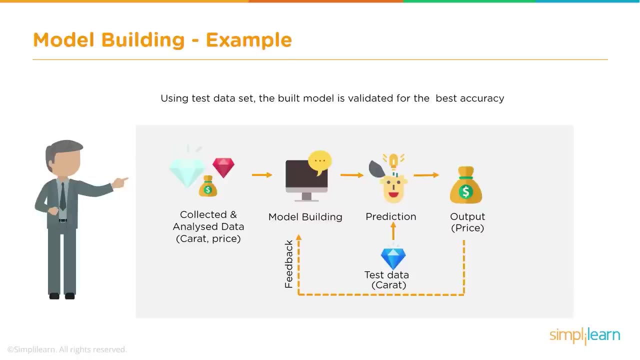 process of this model does. At the end of the training process you have a certain value of m and c and that is used for predicting the values of any new data. that comes All right. So the way it works is we use the training and the test data set to train the model and then validate whether. 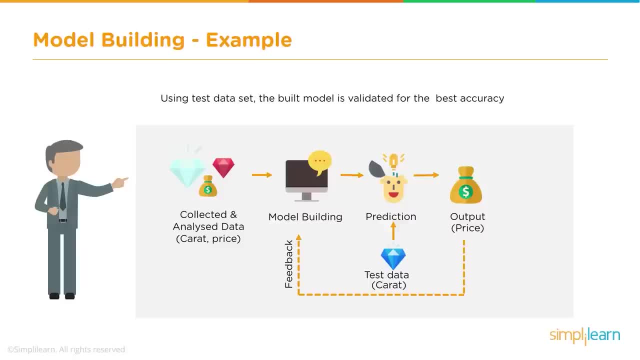 the model is working fine or not, using test data. And if it is working fine, then it is taken to the next level, which is put in production. If not, the model has to be retrained. If the accuracy is not good enough, then the model is retrained, maybe with more data, or you come up with a newer model. 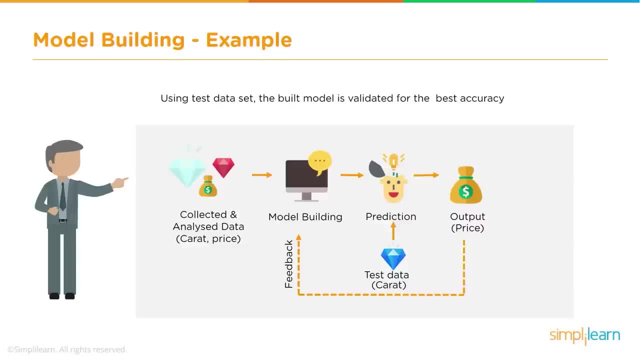 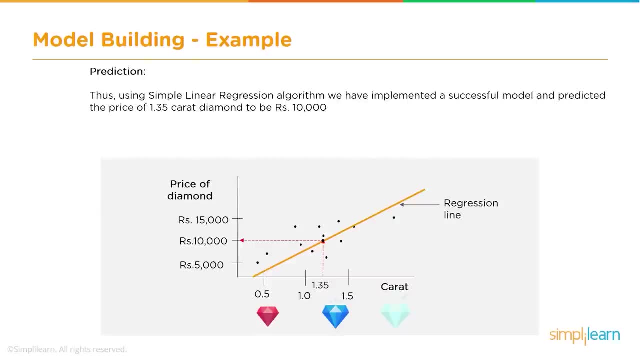 or algorithm, and then repeat the training. So that's how it works. So that's how it works, So it is an iterative process. Once the training is completed- training and test- then this model is deployed and we can use this particular model to determine what is the price of 1.35 carat diamond. 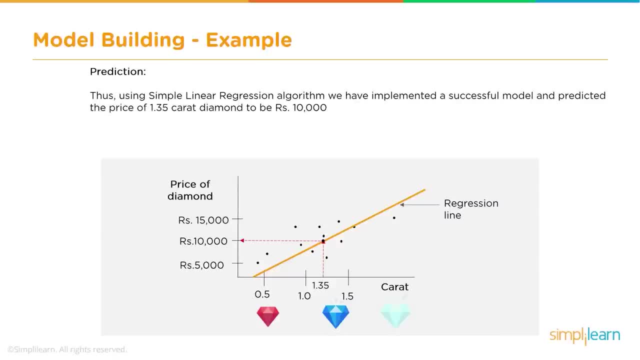 Remember that was our problem statement. So now that we have the best fit for this given data, we have the price of 1.35 carat diamond, which is 10,000.. So this is one example of how this whole process works. 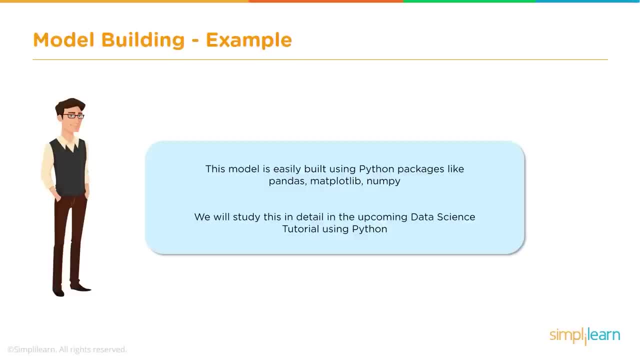 Now, how do we build the model? There are multiple ways. You can use Python, for example, and use libraries like Pandas or NumPy to build a model and implement it. This will be available as a separate tutorial, a separate video, in this playlist. So stay tuned. 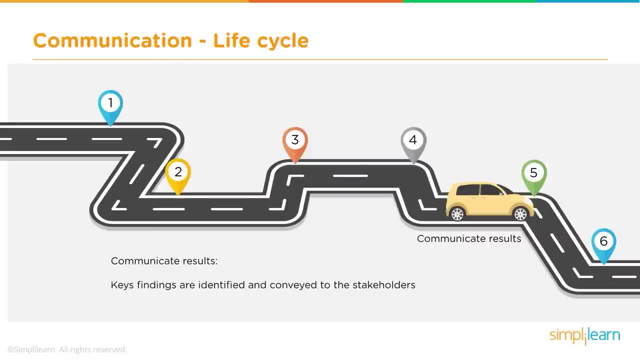 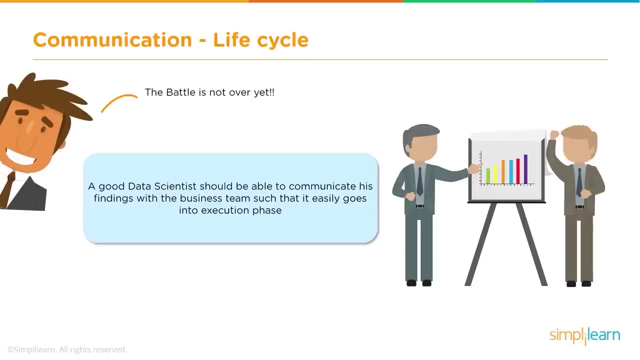 for that. Moving on, once we have the results, the next step is to communicate these results to the appropriate stakeholders. So it is basically taking this results and preparing like a presentation or a dashboard and communicating these results to the concerned people. So finishing or getting the results of the analysis is not the last step, but you need to. 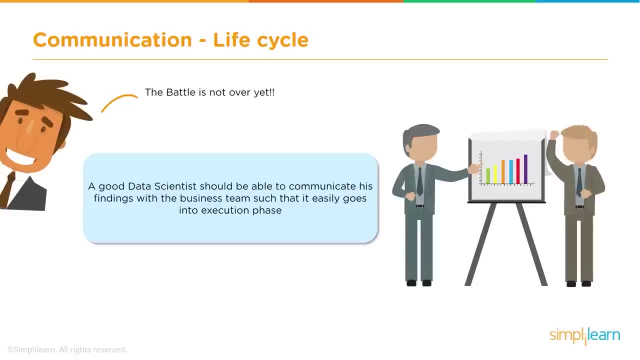 as a data scientist, take these results and present it to the team that has given you this problem in the first place and explain your findings, explain the findings of this exercise and recommend, maybe, what steps they need to take in order to overcome this problem or solve this problem. So that is the pretty much once that is accepted.